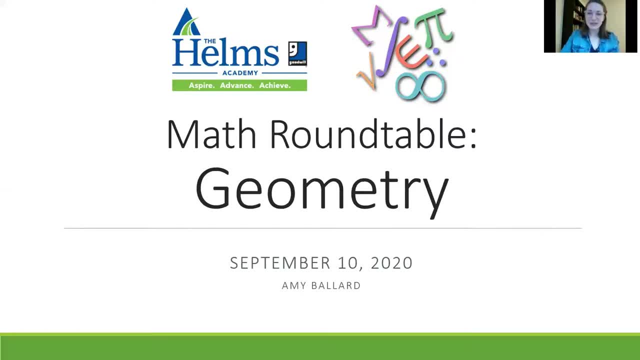 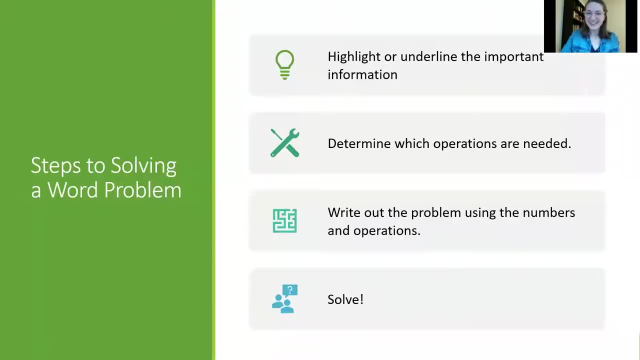 Hi everyone. this is Amy from the Helms Academy, and today we're doing a math roundtable recap for our geometry lesson on September 10, 2020.. So first we went over the steps to solving a word problem, as we always do, and our steps are: 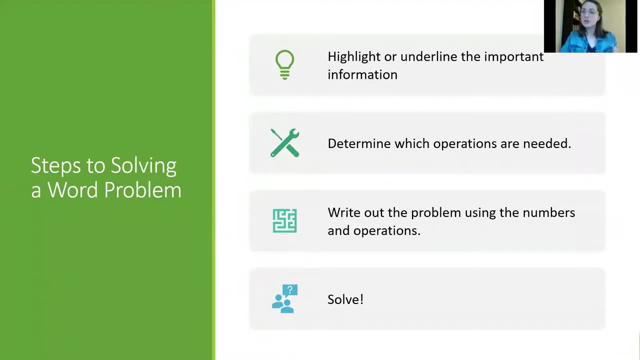 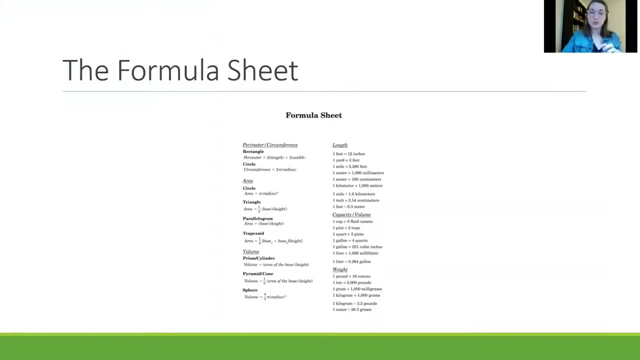 to highlight or underline the important information, to determine which operations are needed and then to write out the problem using the numbers and operations. From there we can solve. So this particular math roundtable is special because we're talking about geometry. When we talk about geometry, it's really important to know your math formula sheet. So the sheet that 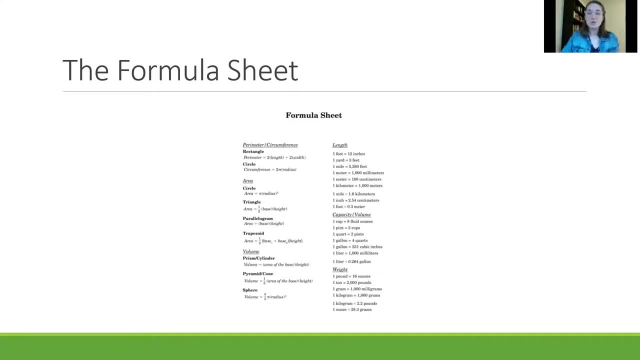 you see on the screen here is for the HiSET exam, and there's also a separate one for the GED exam and a separate one for the TASC exam. You can find them by searching the name of your test and then typing in formula sheet, and they should pop right up on a Google search. 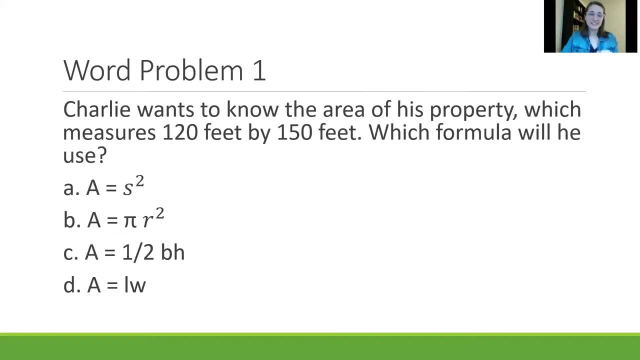 So today, when we're talking about word problem one, it says Charlie wants to know the area of his property which measures 120 feet by 150 feet. Which formula will he use? So what's interesting to me about this problem is they're not asking me to solve, they're asking me which formula will I. 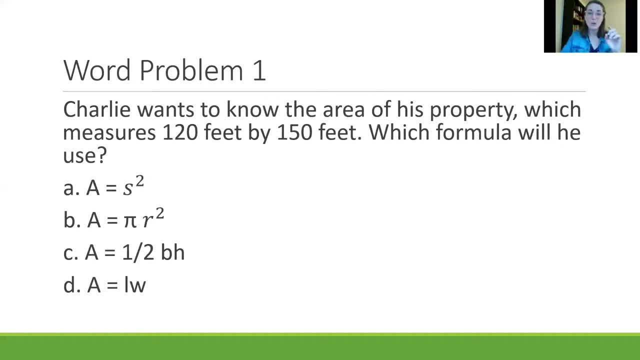 use. So that's why it's also important to look at both what they're asking and also what the options are in the A, B, C and D here. So I'm going to go ahead and type in the A, B, C and D here- multiple choice- because that will help. 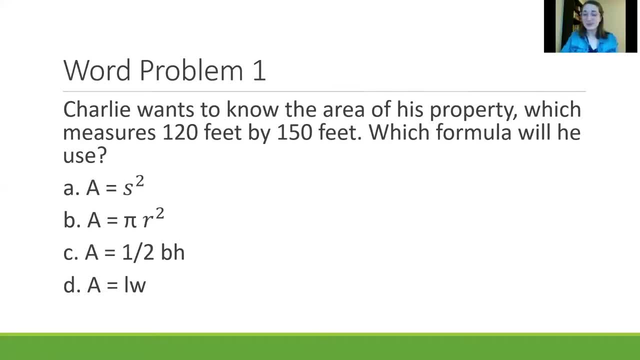 us to narrow down what we're going for. So here I know he wants to know the area, and I see what the area is. It says 120 by 150.. When I see area written that way, it's going to cue in my head. 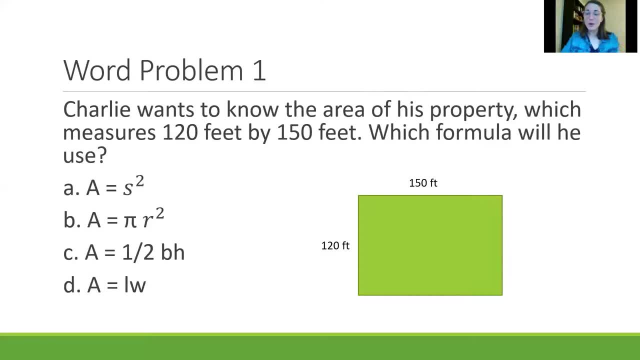 that that has to be a rectangle. So I'm just going to draw a little rectangle so that I know what I'm looking at. So I see 120 by 150 and I see the sides there and that would help me understand. to figure out what formula I'll need. I need to remember what is the formula to use if we're 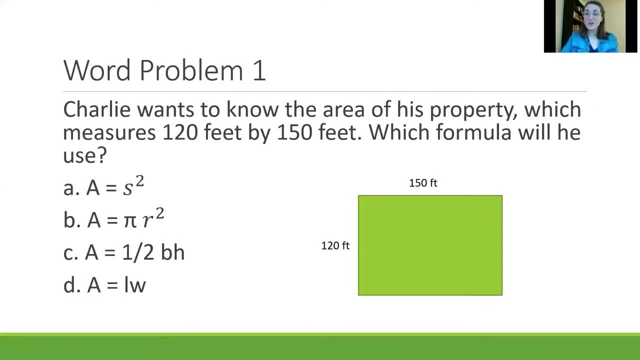 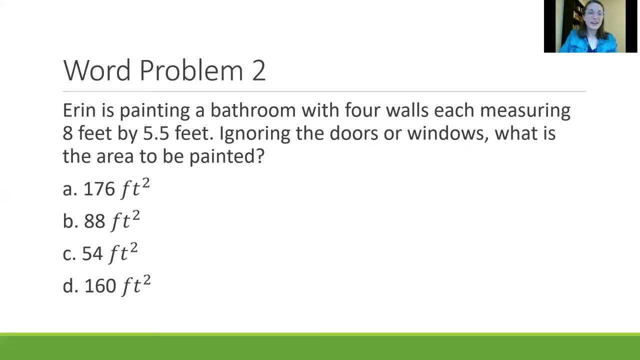 trying to find the area of a rectangle. Well, I know the area for a rectangle is always going to equal the length times the width. So I'm going to look at my options. I see A equals L times W, and that's the correct answer For word problem two. it says Aaron is painting a bedroom with four walls. 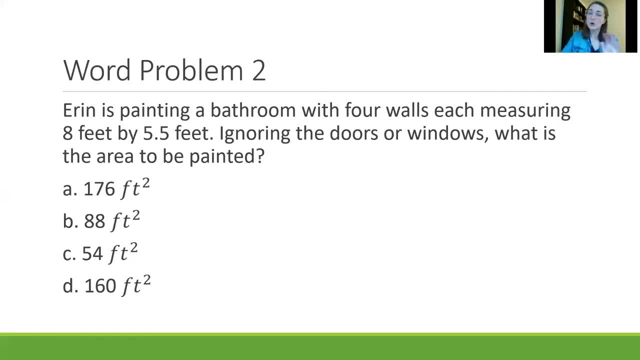 each measuring eight feet by five point five feet, And I say you should call it just the area of the bathroom. So again, the area isn't colour, And what that means is we're drawing a land, So it's alig. Corneline again. 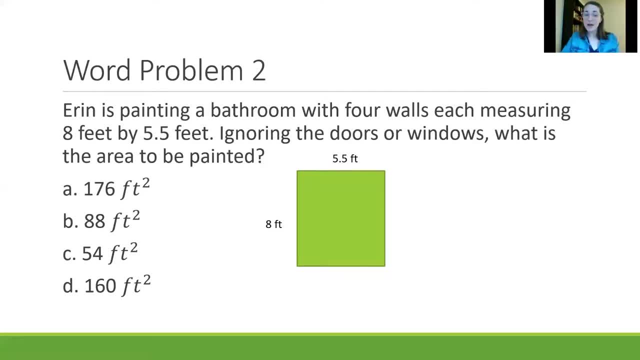 to draw a line like this. So again, the door and windows. What is the area to be painted? 8 feet by 5.5 feet, and that way I can figure out what the area of that wall is. Now, it's not just that, though. I also need to do that times 4, because we have 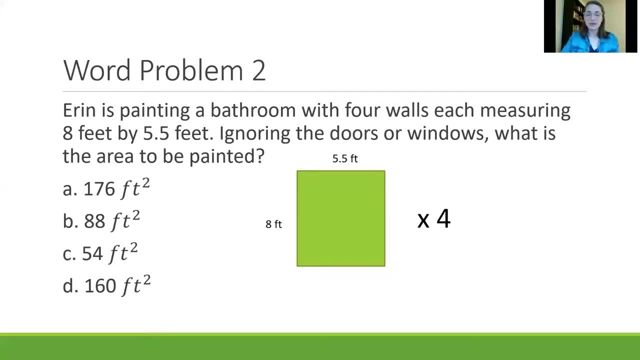 4 total walls that are that same area. So here we're gonna do 8 times 5.5, because that will get the area of one wall. but then we need to multiply again times 4 and we put all that together we get 176 feet. squared Area will always be. 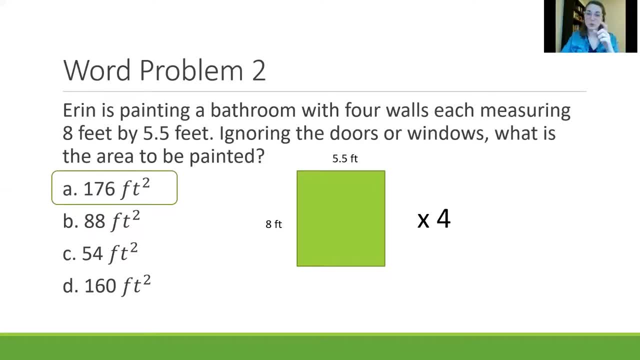 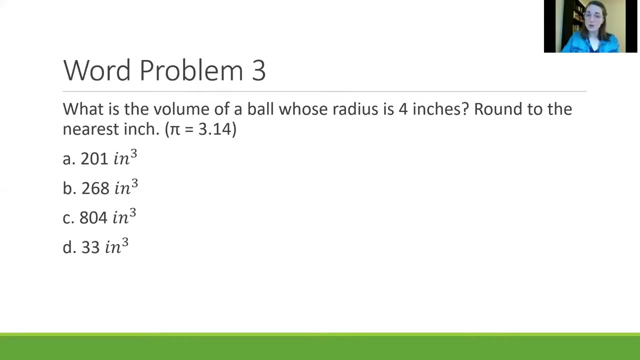 measured in feet squared or whatever. the unit is squared with the two above it as an exponent. So remember, if you're writing the answer for area, to include that piece. For word problem 3 it says: what is the volume of a ball whose radius is 4 inches, Round to the nearest inch? 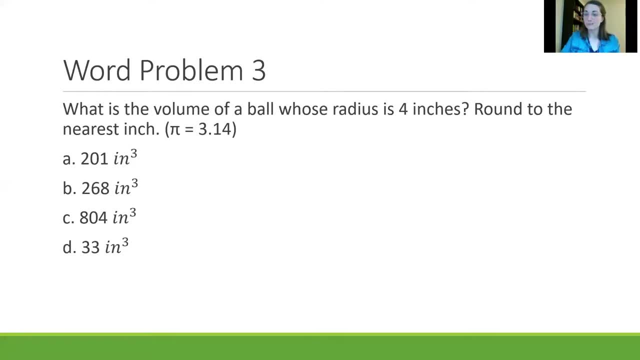 And it tells us that pi equals 3.14.. That's a clue to me, because if I see pi equals 3.14, then I bet I'm gonna be using a formula. So I'm gonna go to my formula sheet and see what it says. Here's the section of the HiSET formula. 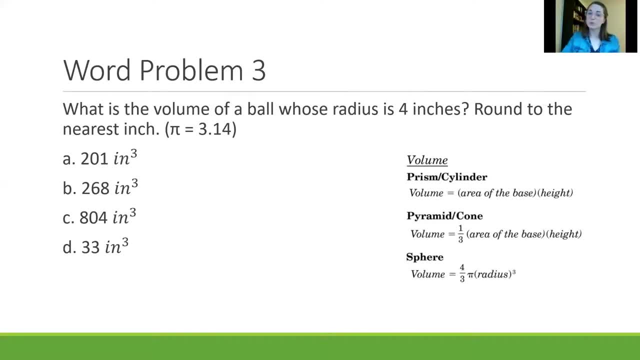 sheet that has to do with volume And you can see it shows volume for a prism or a cylinder, a pyramid or a cone or a sphere. So I need to figure out here what I need. It says a volume of a ball. Well, a ball in general is the volume of a ball. 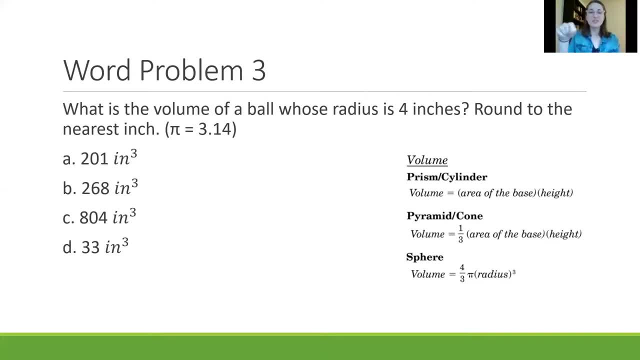 So I'm going to use the formula that you see there. So I'm going to use the formula that you see there. Volume equals 4 thirds times pi, times radius cubed. So when I rewrite that, I'm going to keep the 4 thirds, I'm going to replace pi with 3.14, as it told me to do. 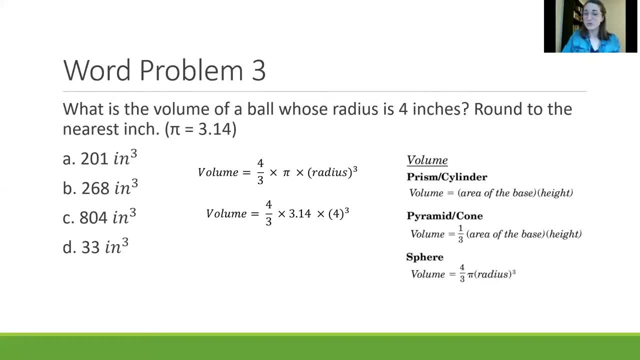 And then I need to fill in what my radius is, which is 4.. And we need to keep the cubed there as well. Now, using the order of operations, I am going to do my exponents first. Everything in parentheses is just a single number, so I can skip right to the exponent step. So 4 cubed or 4 times 4. 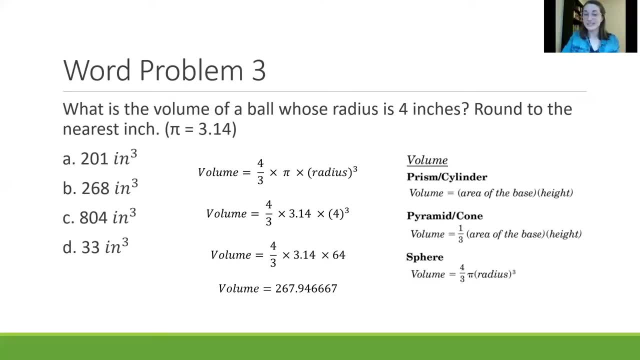 times 4 is 64. And you can see. I replaced that on the third line there. So now I just need to multiply across. And when I multiply across I see that the volume is 267.946667.. Well, that's not my final answer, because I need to round. 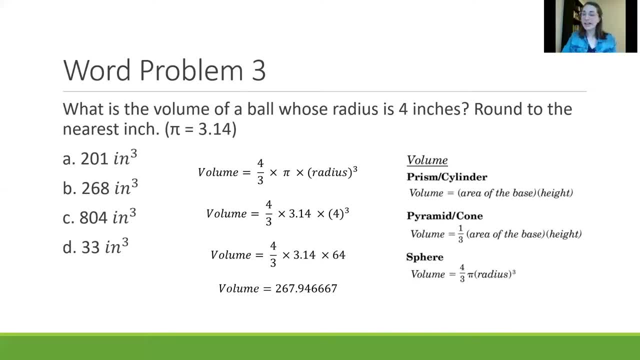 to the nearest inch. So because it has a 9 after that decimal place, the decimal point, then I'm going to round up to 268.. And the way I write this is in inches cubed, So you'll see that. inches to the third and our final answer is B Word. 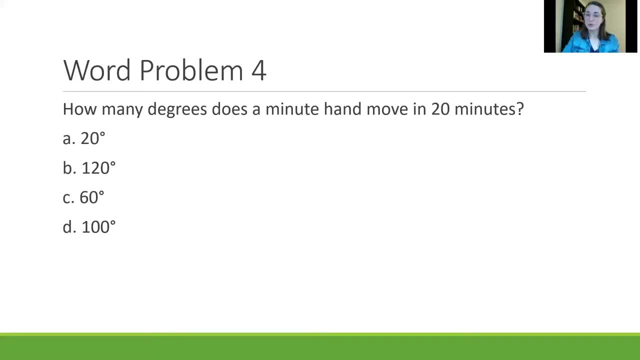 problem 4 says: how many degrees does a minute hand move in 20 minutes? So when I think about this, I'm thinking degrees. Are we talking about degrees in the about temperature here? Well, no, this isn't about temperature. It talks about a minute hand and 20. 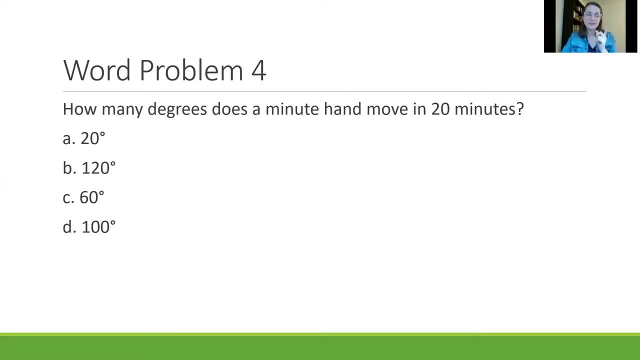 minutes. So I'm getting the image of a clock and I'm guessing if we're talking about degrees, it has to do with angles on a clock. So this is wondering: in 20 minutes, how many degrees does this move? Well, I'm going to pull up some visuals. These visuals would not be included on the text. 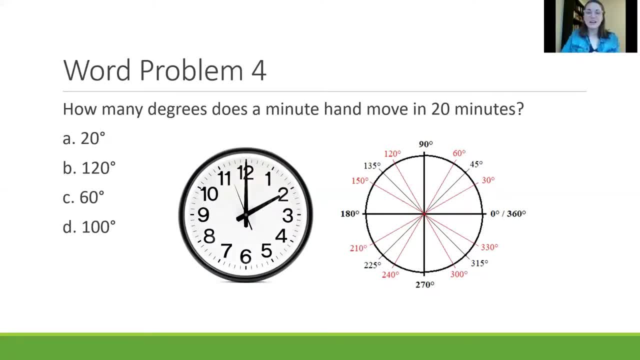 but test. but they will be helpful for us today. So we can see the degrees on the right side of a circle and you can think about this logically right. Think of a 90 degree angle is always that right angle. there You can think about if you turn from one direction to another. 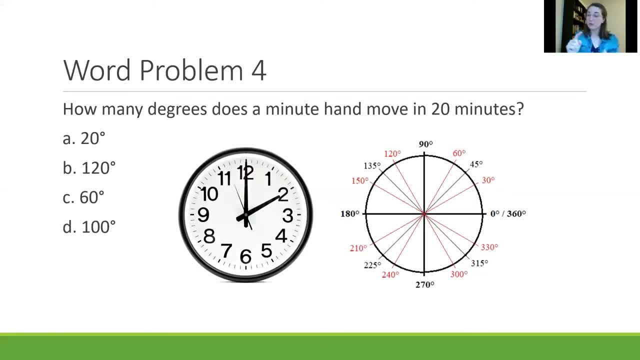 you might do 180 degree turn or if you do a full circle around, that's a 360. So some of these things you've probably heard before or worked with before, so we can keep that in mind when we're solving this problem. So think about 20 minutes on a clock. 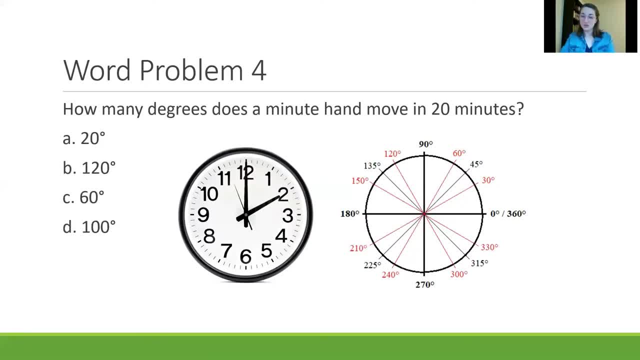 and what degree that would be when we look at the degrees here. Now again, you won't have these visual aids, so while you can maybe sketch these out and take a good guess, the best way to solve would actually be to make a proportion. So think about it this way: How many total degrees do we? 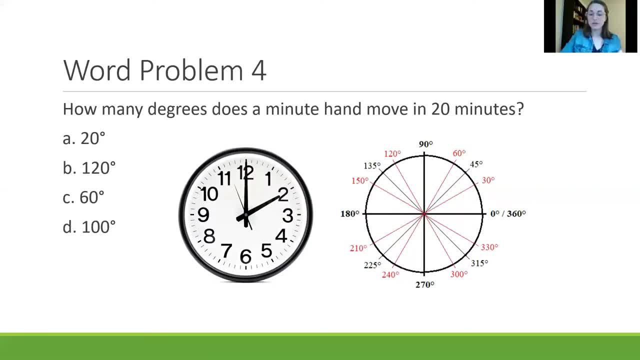 have on a clock total minutes 60. So if we want to figure out what 20 out of 60 minutes is in terms of degrees, I can set it up like a proportion. 20 minutes out of 60 minutes on a clock is equal to. 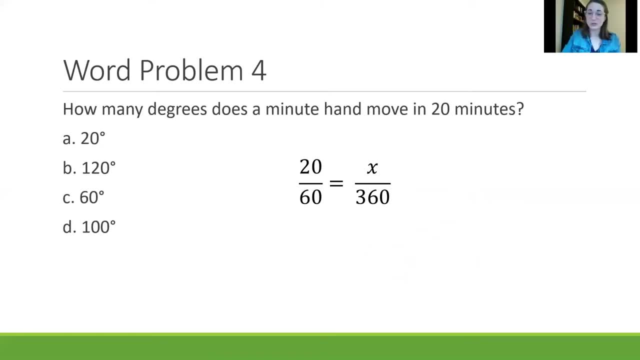 how many degrees out of 360 degrees on a full circle. So to solve that we're going to cross, multiply our 20 times 360 and then we're going to divide by our other number, which is 60. So in our multiply we get 7200 and we divide that by 60 to get our answer of 120. so the 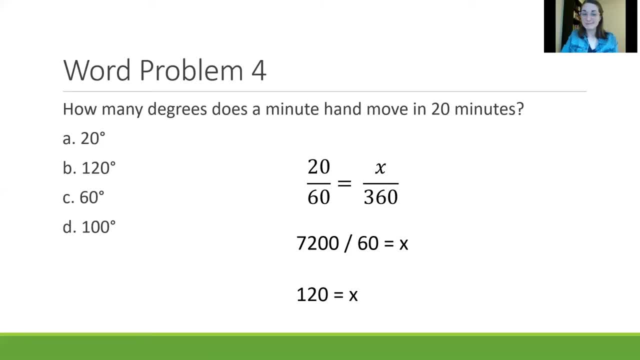 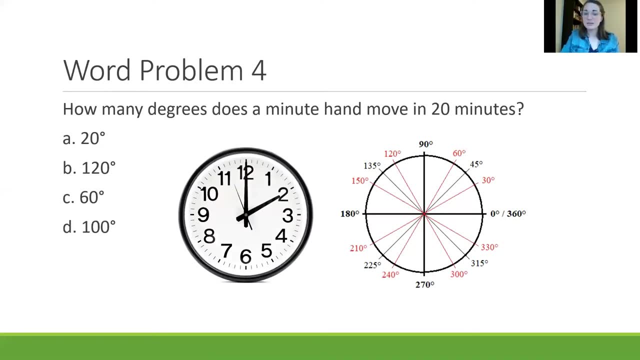 final answer: there is 120 degrees. now I want to go back just to look at our clock and our degrees. you can think about it simply. it's just thinking: okay, 15 minutes. right, you know, 15 minutes would be going from the 12 to the 3. that 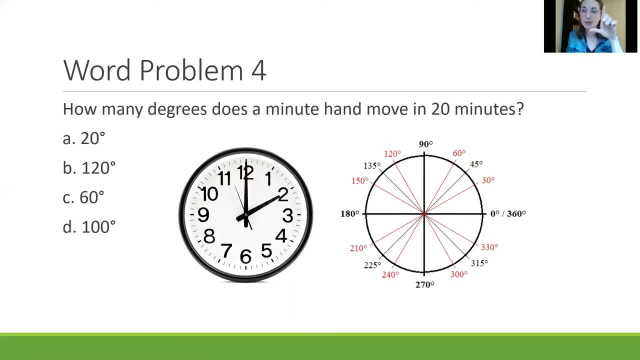 would be a right angle. so we know that's 90 degrees there, so 20 minutes is going to be more than that. so right away I can root out a and C, 20 degrees and 60 degrees, because they don't even meet the minimum of 90 degrees which I could. 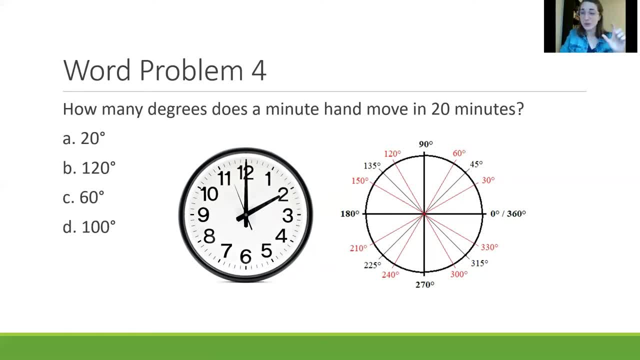 guess pretty quickly so we could get it down to two answers very quickly. and if you were in a rush and try to finish up some answers for a test because you were running out of time, then I would suggest using that technique as a way to at least 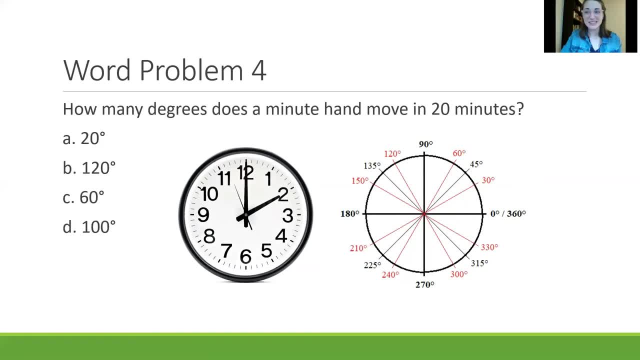 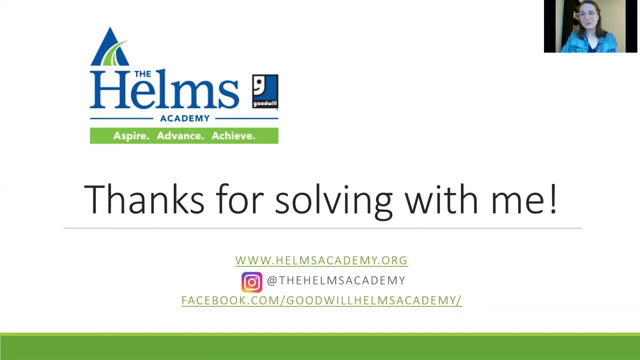 you know, get the answer right and then you can go back and look at your clock. just limit yourself down to a few options and take the best guess from there. thank you so much for solving with me today and checking out these problems. I hope you learned something new and that you'll subscribe to our YouTube.